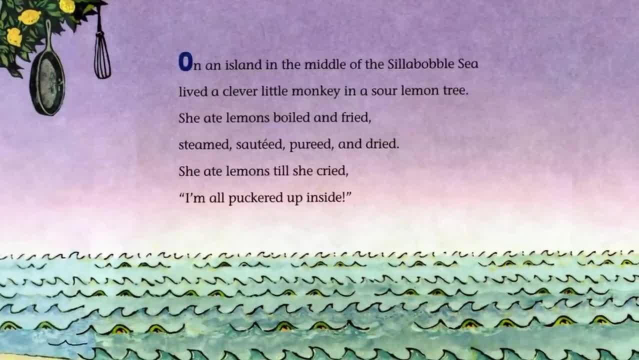 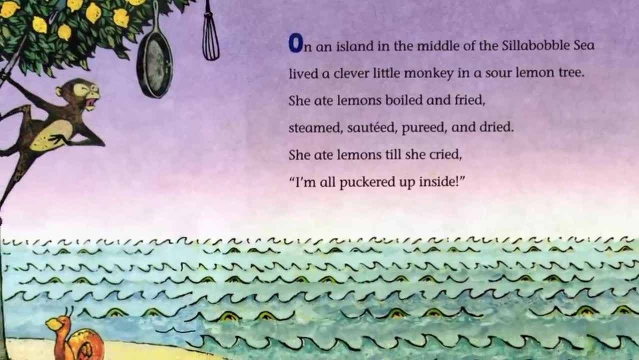 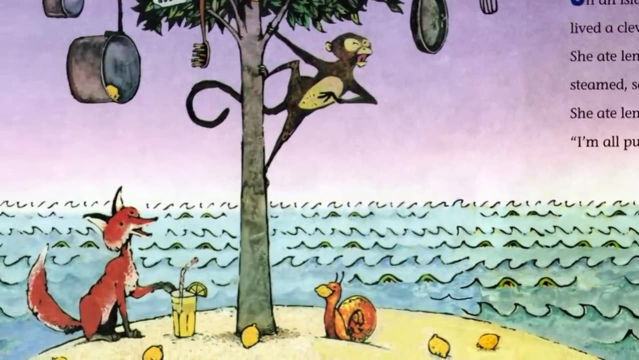 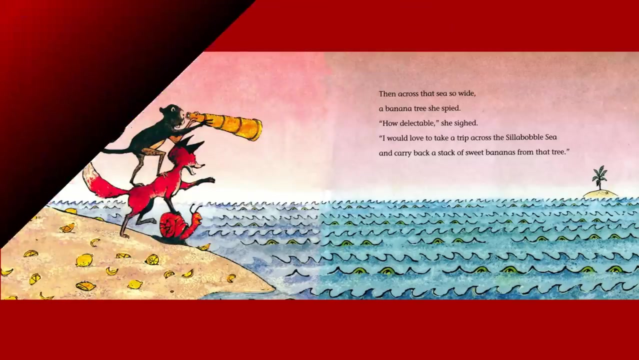 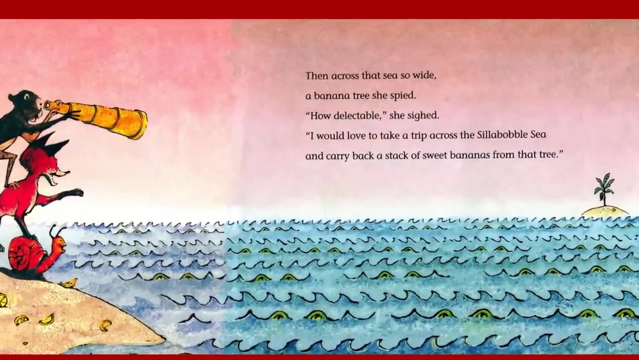 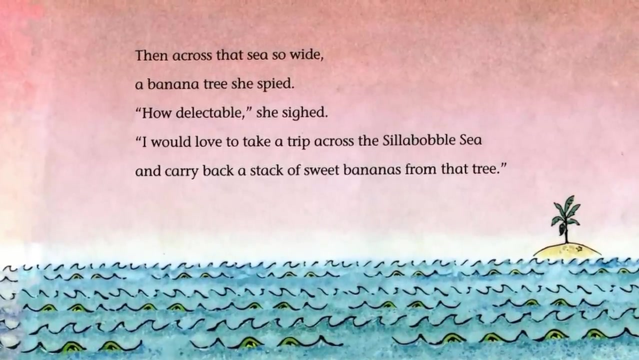 flower-lemon tree. She ate lemons boiled and fried, steamed, sauteed, pureed and dried. She ate lemons till she cried. I'm all puckered up inside. Then, across that sea so wide a banana tree, she spied How delectable. she sighed I would love to take a trip across. 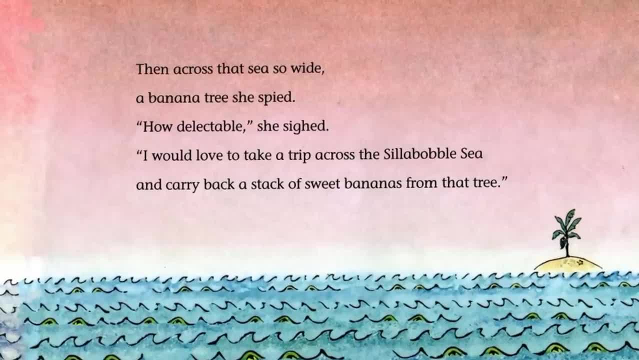 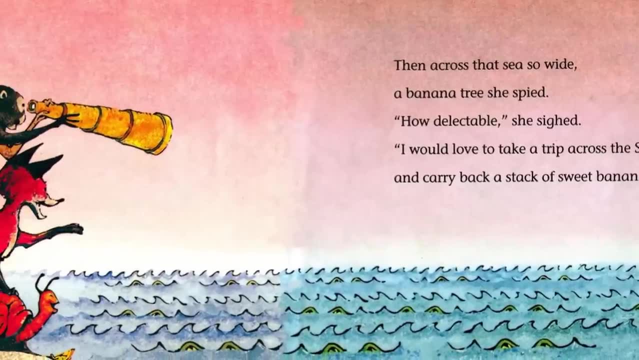 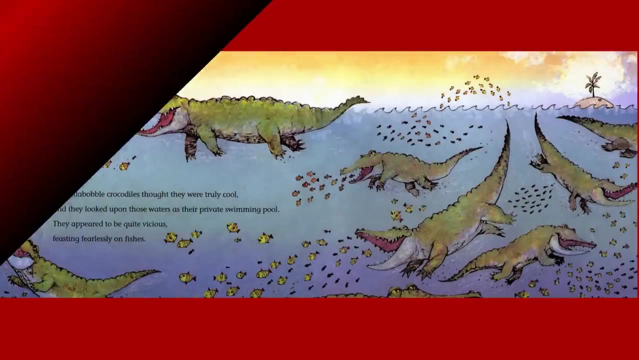 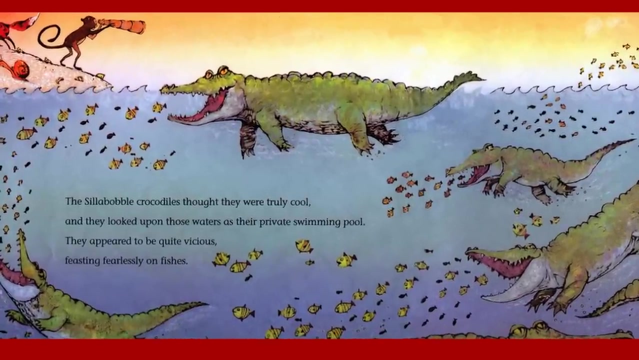 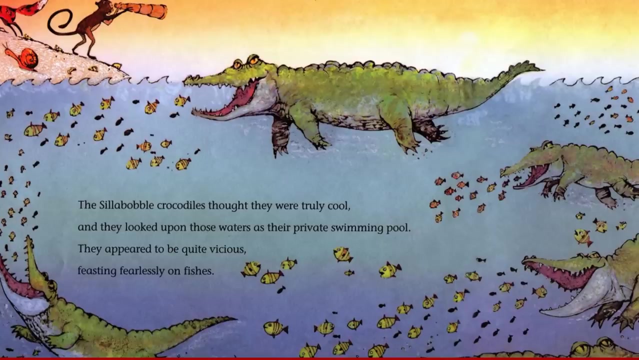 the Silla-Babble Sea and carry back a stack of sweet bananas from that tree. The Silla-Babble crocodiles thought they were truly cool and they looked upon those seas as their private swimming pool. They appeared to be quite vicious, feasting fearlessly. 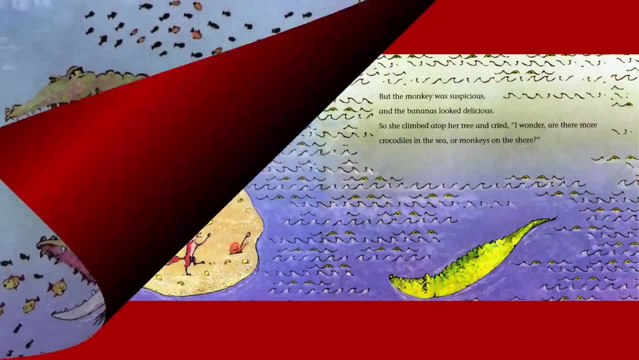 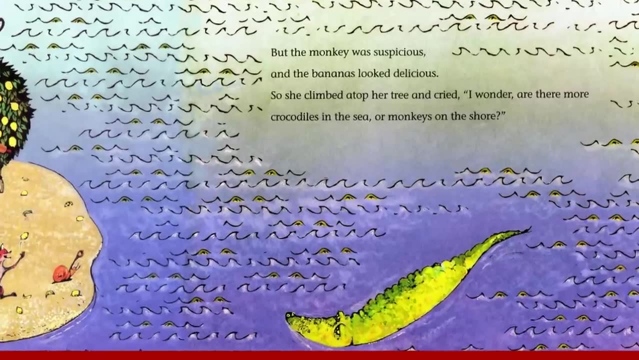 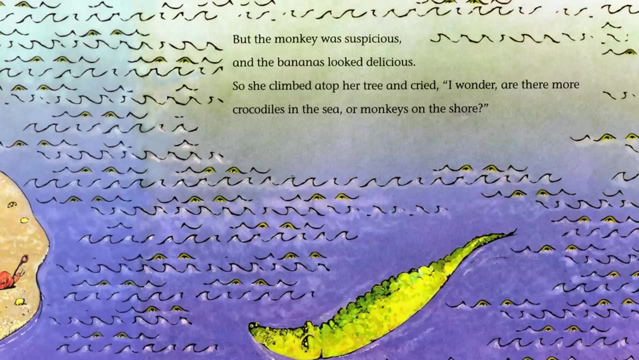 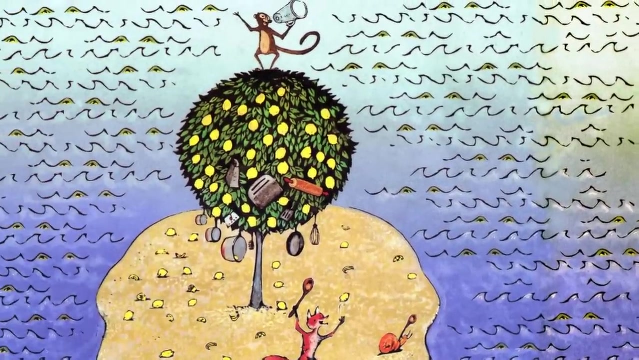 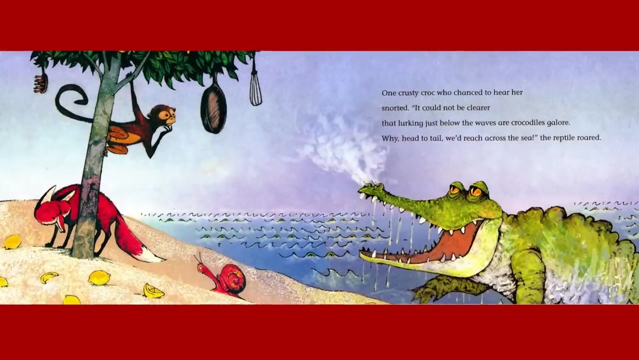 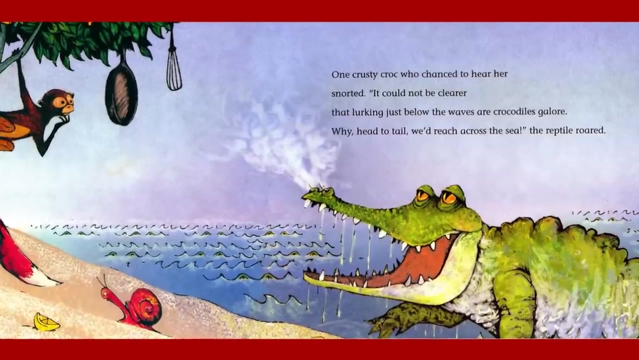 on fishes. But the monkey was suspicious and the bananas looked delicious, so she climbed atop her tree and cried: I wonder, are there more crocodiles in the sea or monkeys on the shore? one, Krusty Kruk, who chanced to hear her, snorted. it could not be clearer that. 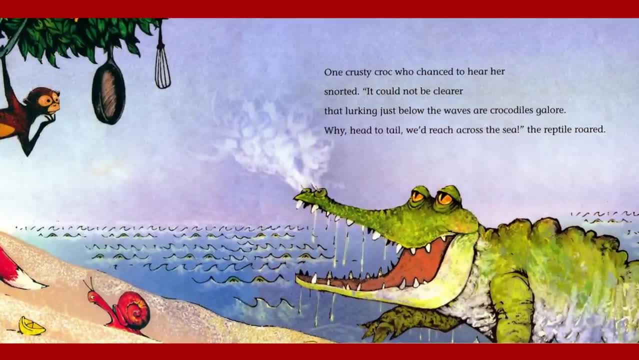 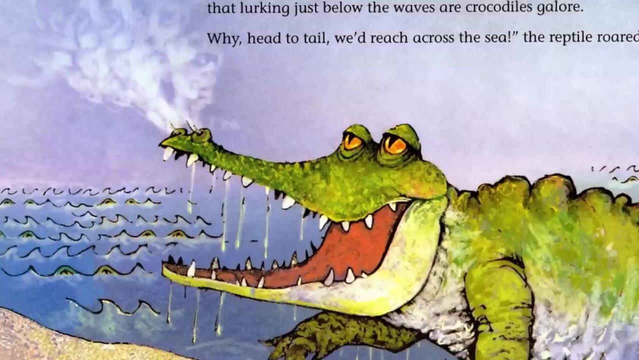 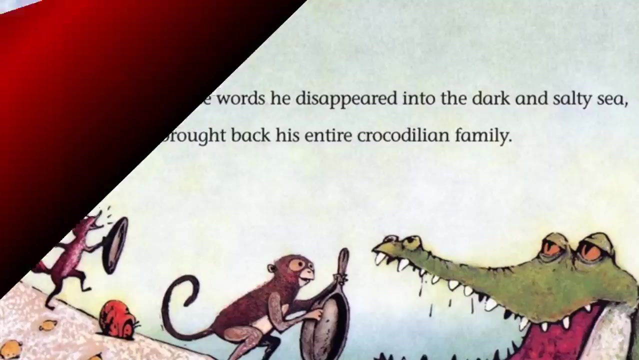 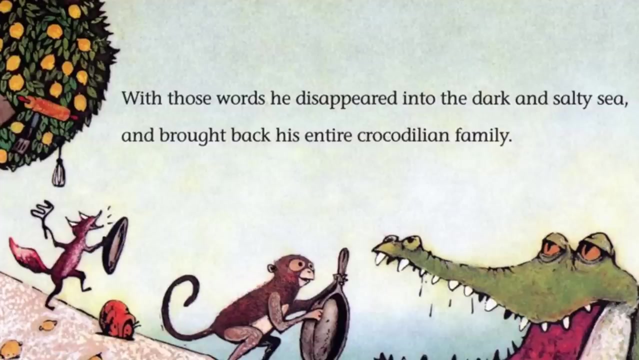 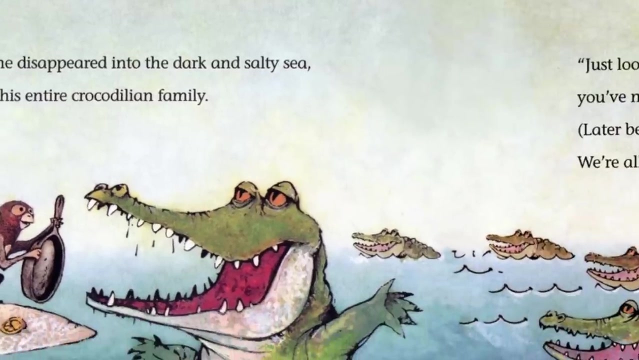 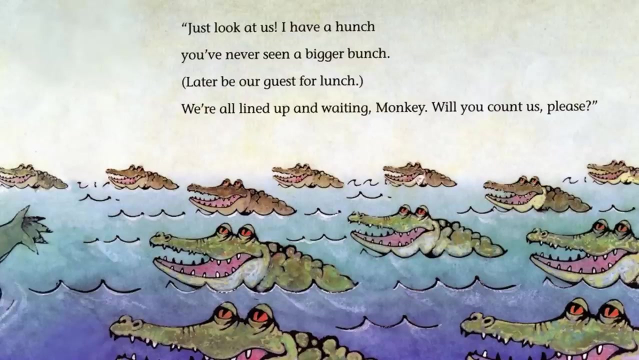 lurking just below the waves, our crocodiles galore, why? head to tail, we'd reach across the sea. the reptile roared. with those words, he disappeared into the dark and salty sea and brought back his entire crocodilian family. just look at us. I have a hunch. you've never seen a bigger bunch. Later, be our guest, for. 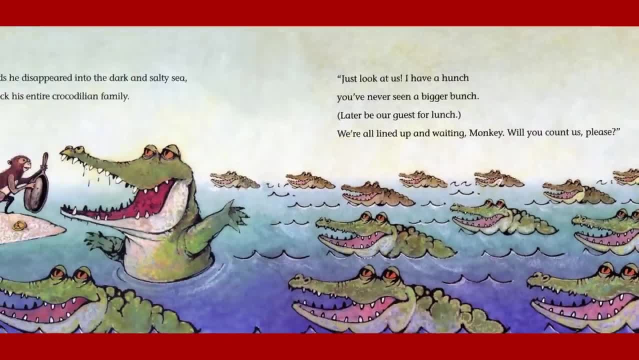 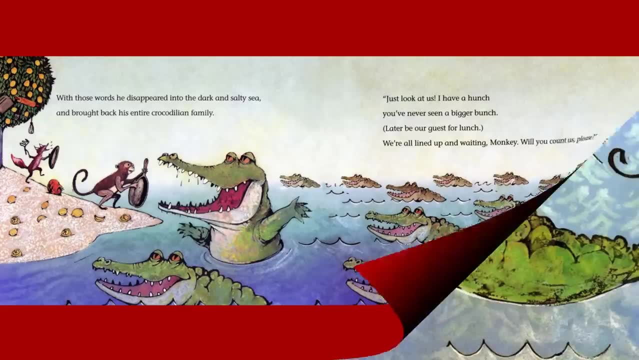 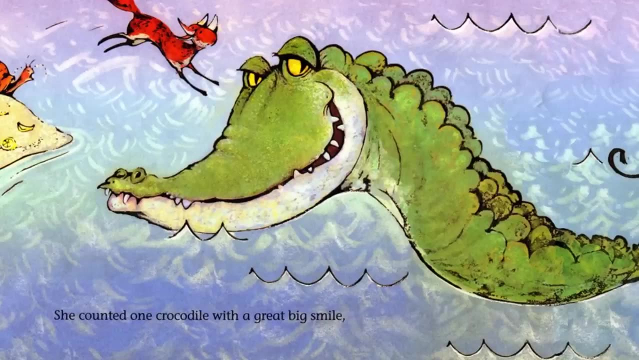 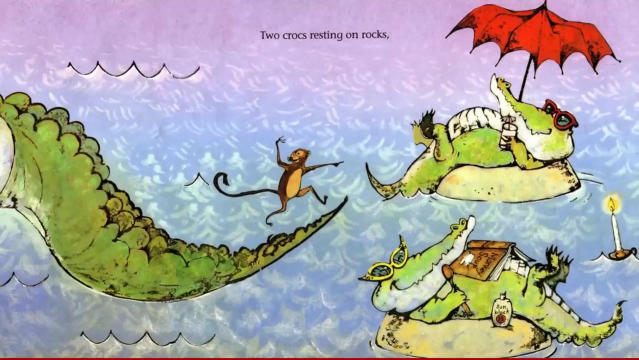 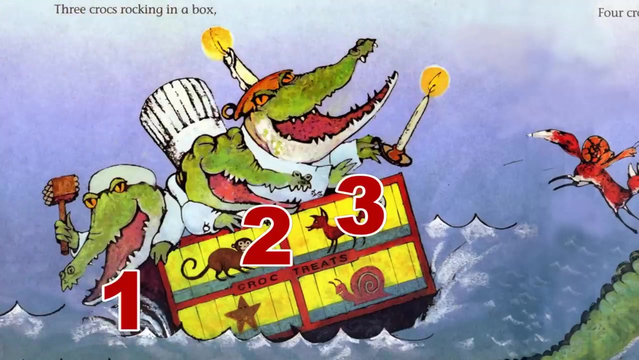 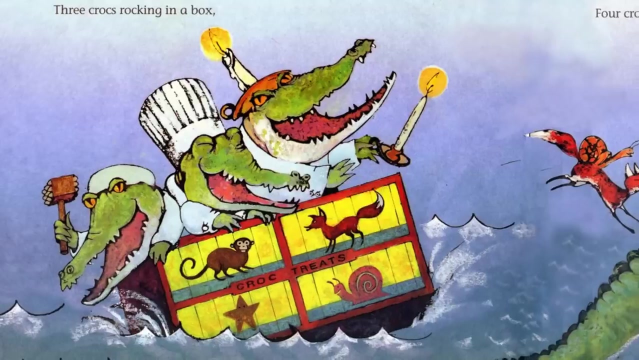 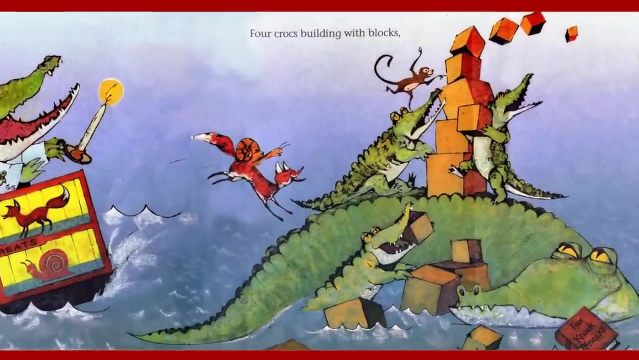 lunch. We're all lined up and waiting. monkey, Will you count us please? She counted One crocodile with a great big smile, Two crocs resting on rocks, Three crocs rocking in a box, Four crocs building with blocks. 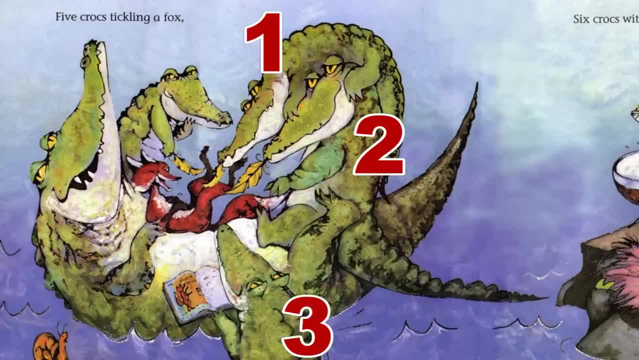 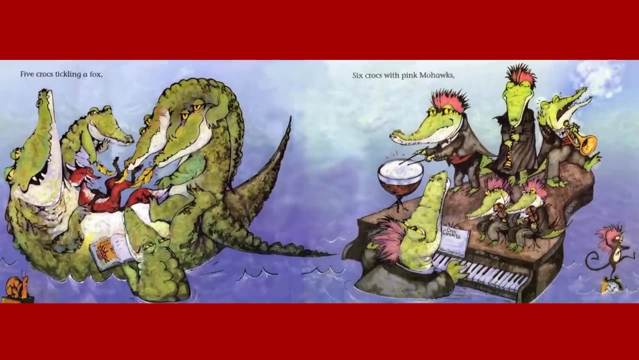 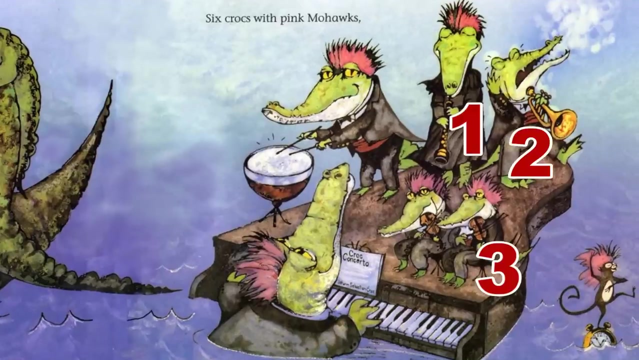 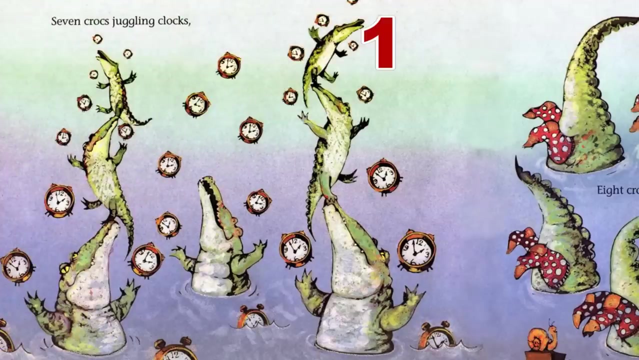 Five crocs tickling a fox, Six crocs with pink mohawks, Six crocs with pink mohawks, Seven crocs juggling clocks. I have a hunch. you'll never see a bigger bunch Later. be our guest for lunch. 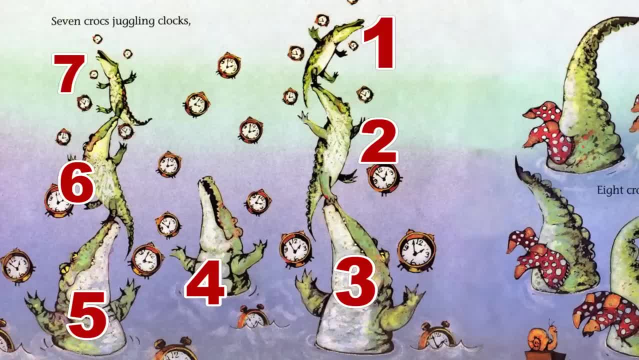 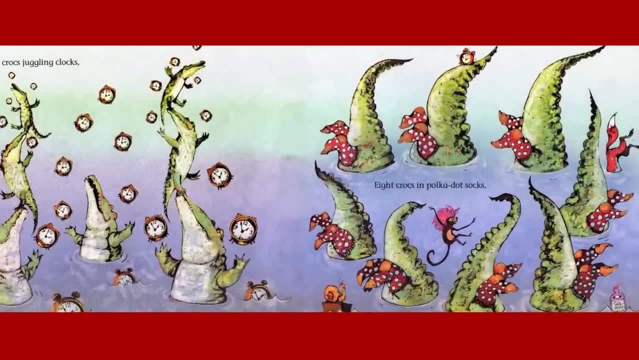 We're all lined up and waiting. monkey, Will you count us please? She counted One crocodile with a great big smile, Two crocs resting on rocks, Three crocs with pink mohawks, Six crocs juggling clocks. 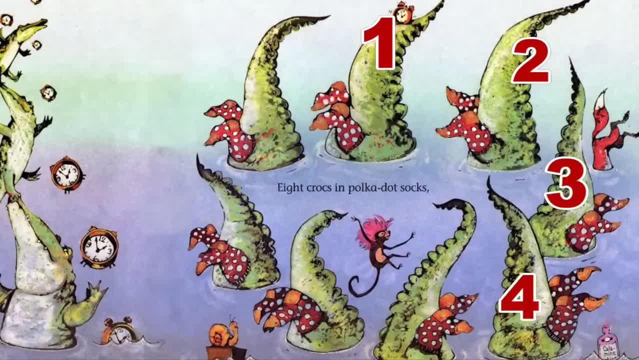 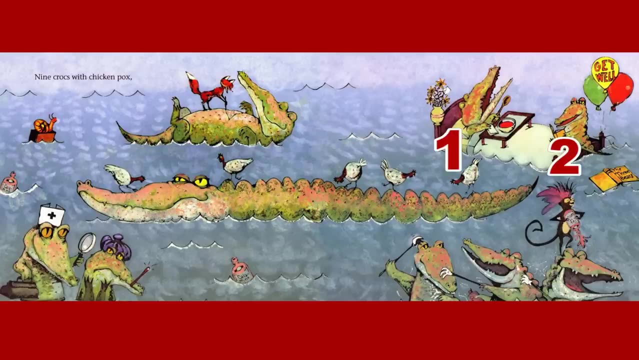 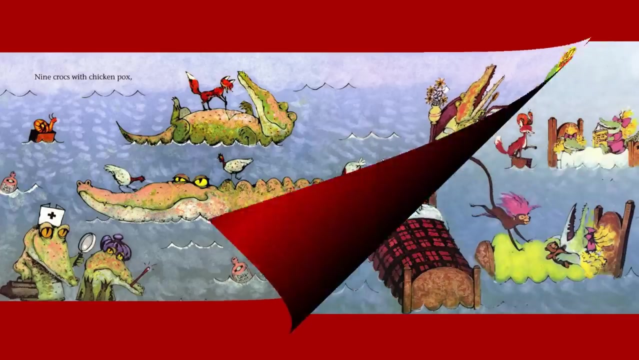 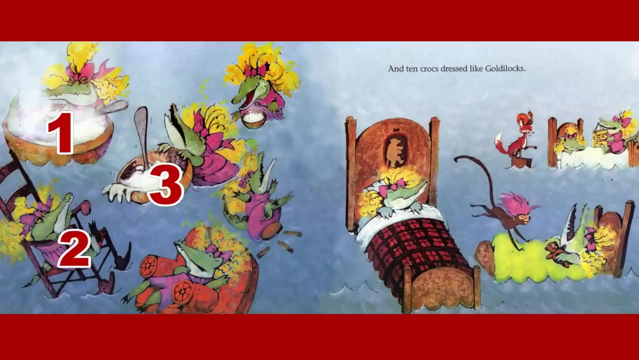 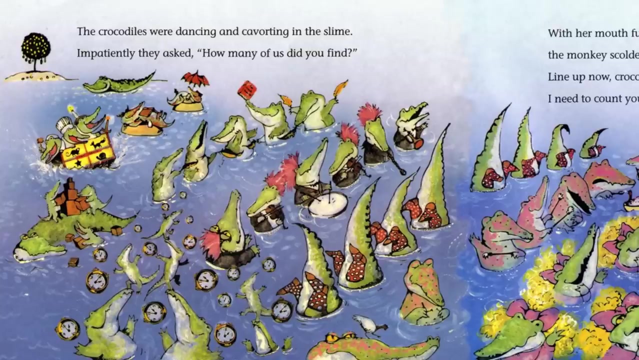 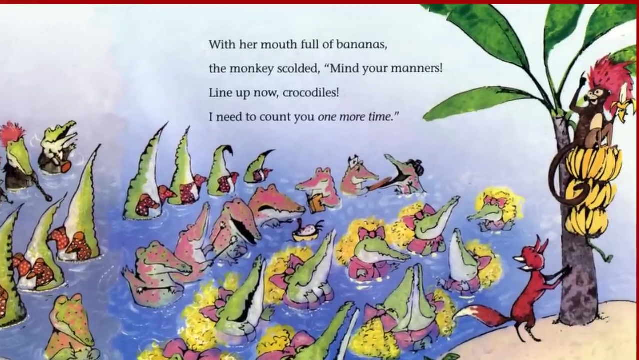 Crocs in polka dot socks, Nine Crocs with chicken pox And ten Crocs dressed like Goldilocks. The crocodiles were dancing and cavorting in the slime Impatiently. they asked: How many of us did you find With her mouth full of bananas? 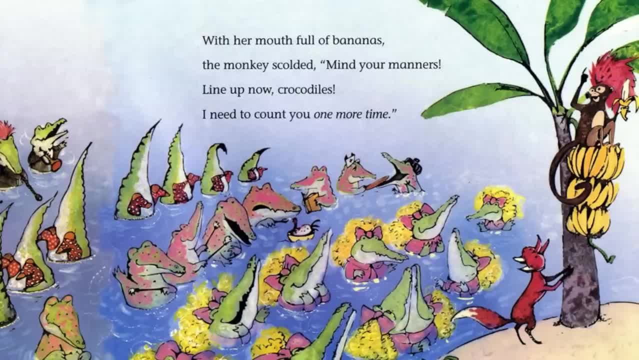 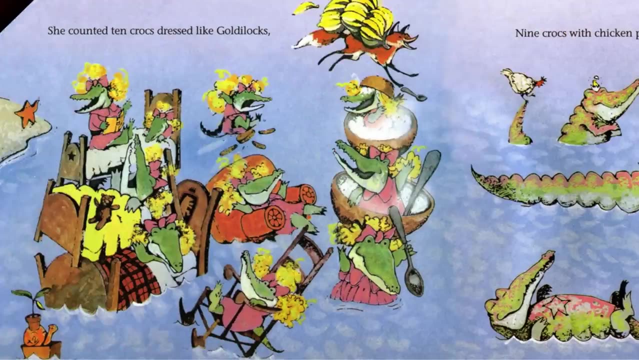 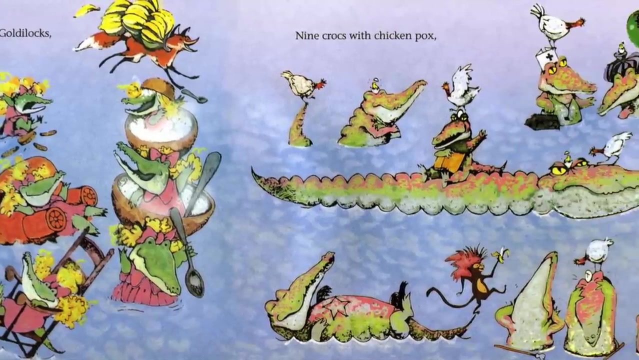 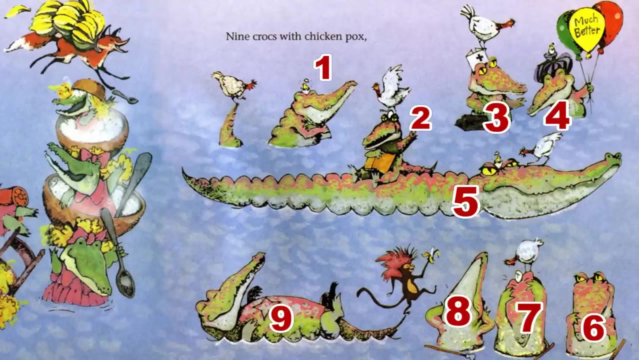 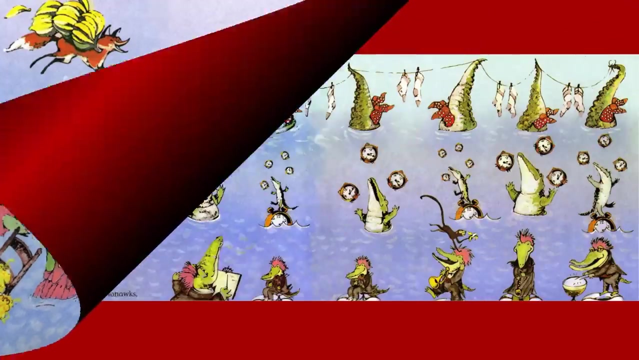 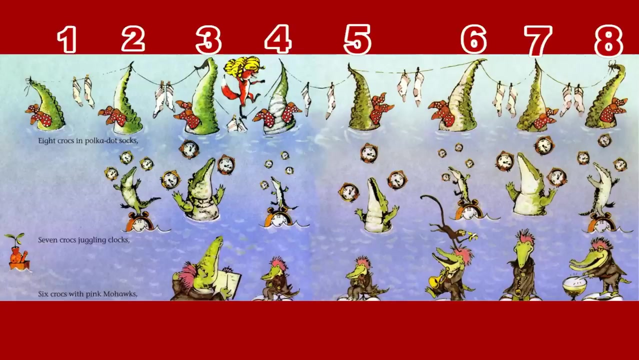 The monkeys scolded. Mind your manners. Line up now, crocodiles. I need to count you one more time. She counted Ten Crocs Dressed like Goldilocks, Nine Crocs with chicken pox, Eight Crocs in polka dot socks And seven Crocs. 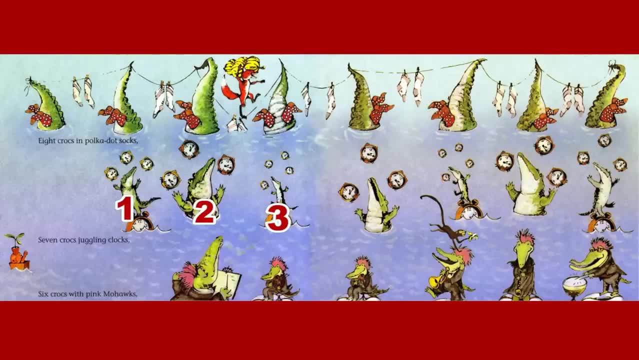 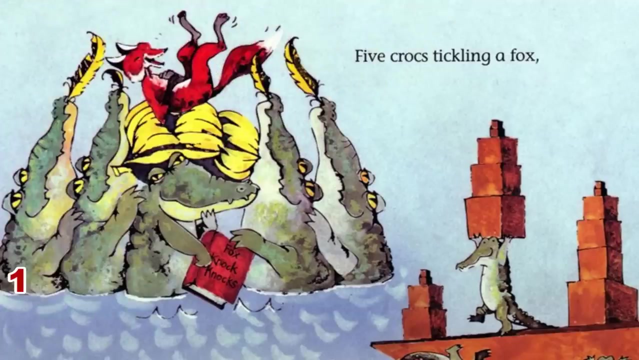 Dressed like Goldilocks, balance The man AP And her face. 13 Crocs, Seven Crocs Juggling clocks, 6 Crocs With pink mohawks, Five Crocs Tickling a fox, Three Crocs. Here are some Likeoman And ה� Premium questeos. 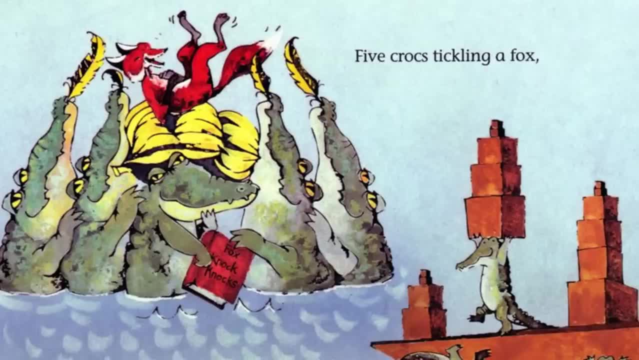 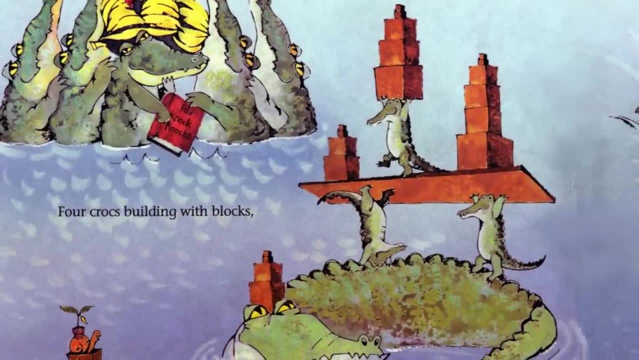 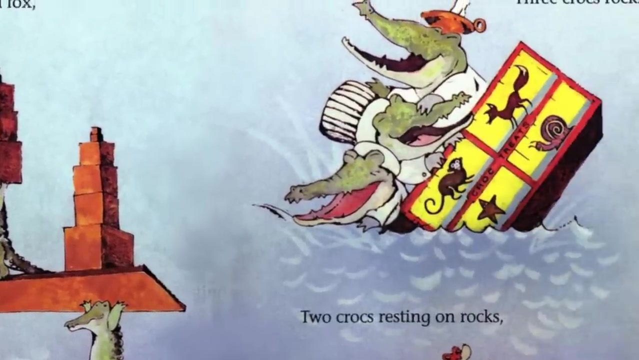 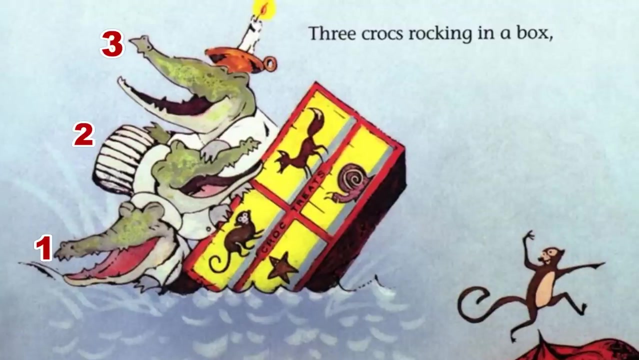 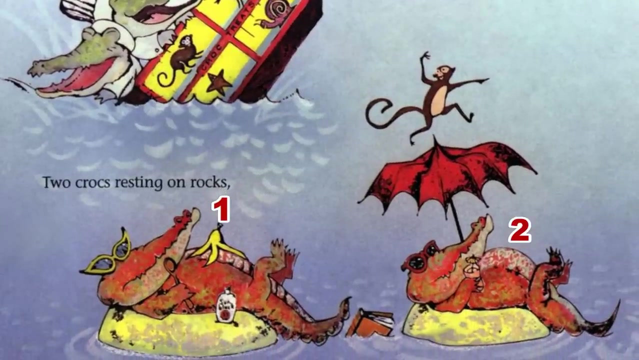 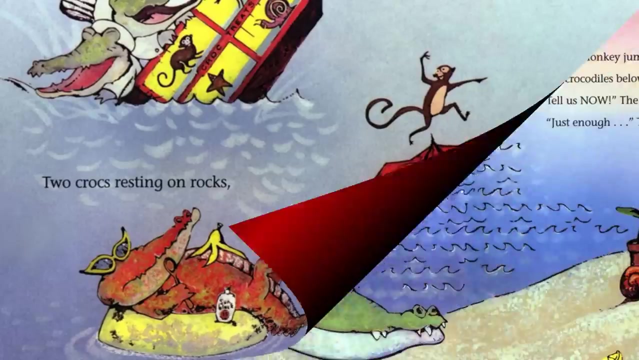 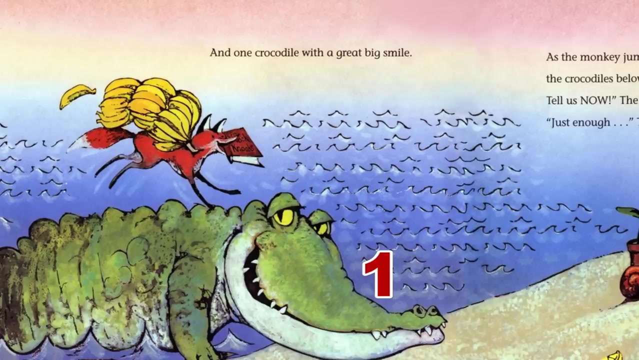 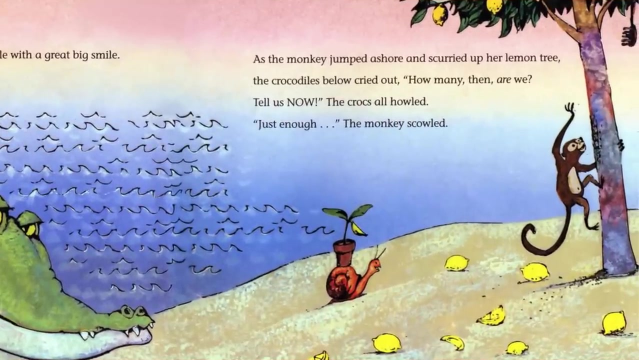 Make you laugh. Four crocs building with blocks, Three crocs rocking in a box, Two crocs resting on rocks, Two crocs resting on rocks And one crocodile with a great big smile As the monkey jumped ashore and scurried up her lemon tree. 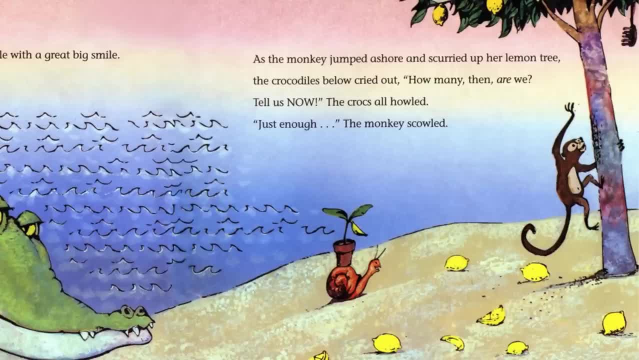 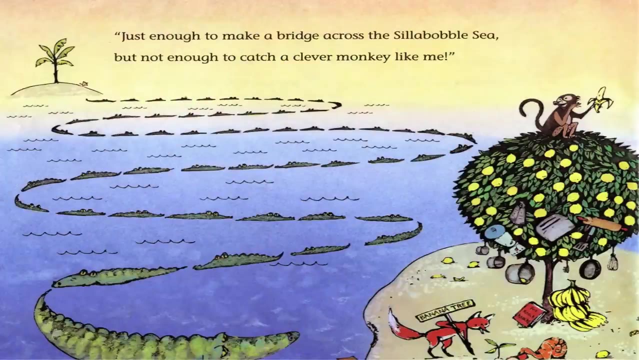 The crocodiles below cried out. How many then are we Tell us now? The crocodiles all howled Just enough. The monkey scowled. Just enough to make a bridge across the Zillababble Sea, But not enough to catch a clever monkey like me. 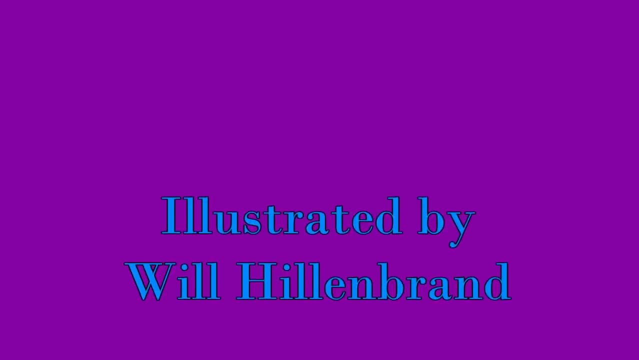 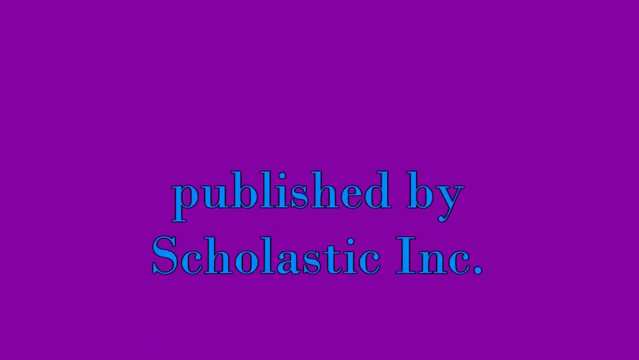 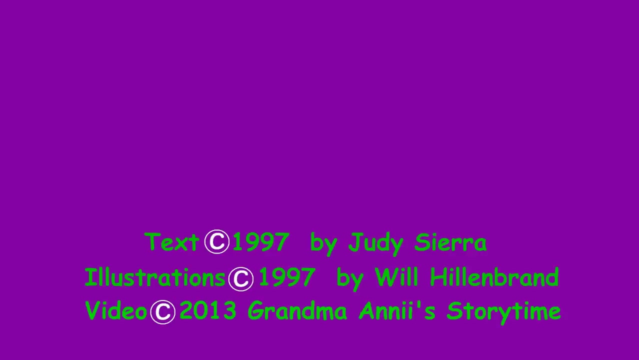 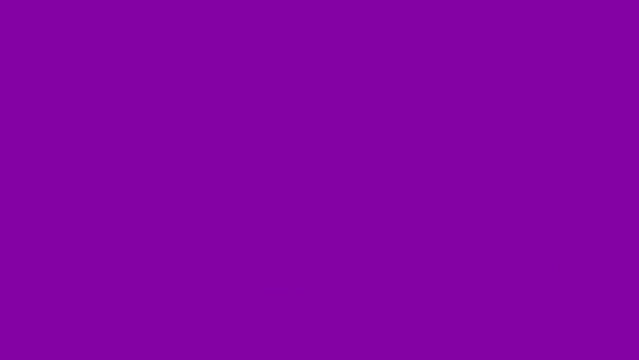 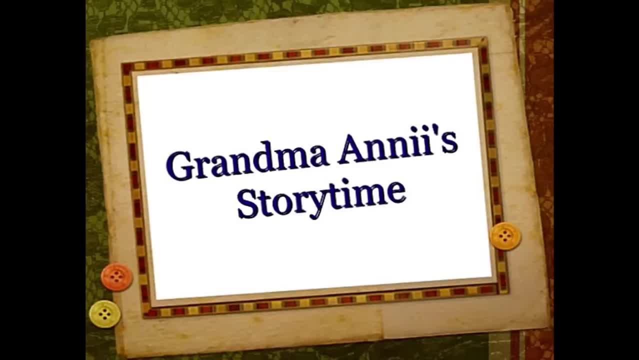